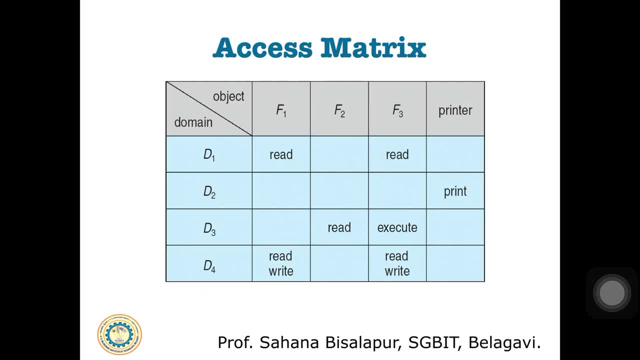 read operation. So a process executing in domain D4 has the same privileges as domain D1, as the process in domain D1, but with one extra operation here, that is write operation. So here, as we can see in the diagram, D4 is having for F1 file read, write operations can be performed and for F3 also there are read. 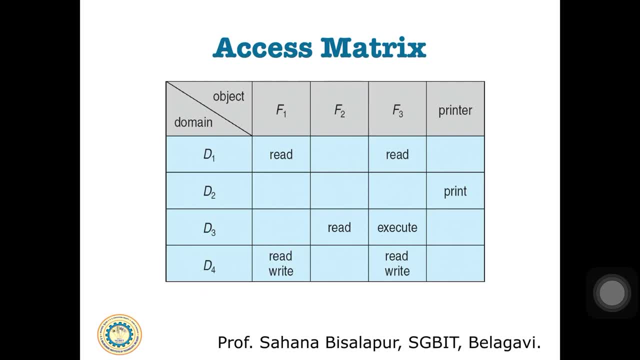 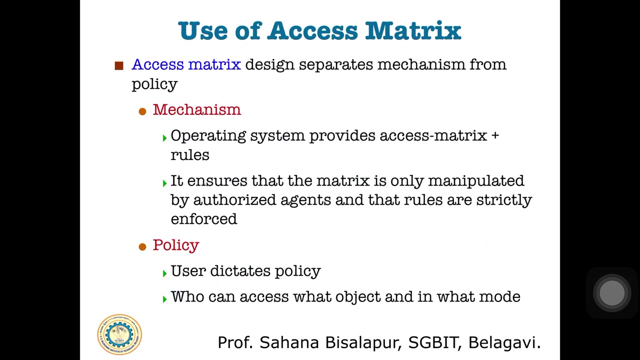 write access writes given for this particular file. So here we are also having a printer as one object here. So here only the printer can be accessed by the process which is in domain D2.. We also have the access matrix Providing some mechanisms and policies here. So these mechanisms are specifying various policies. 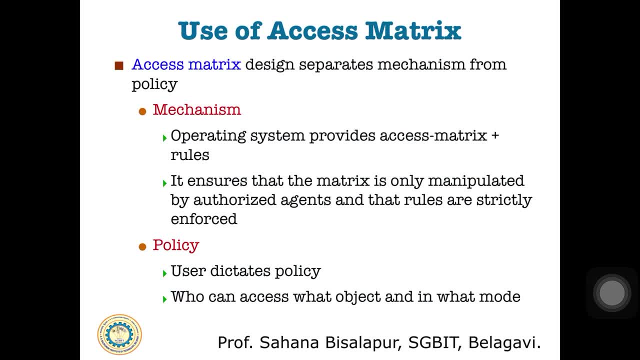 So the mechanisms consists of implementing the access matrix and ensuring that the meaning of this access matrix, whatever we are supposed to have here, the meaning of that- will be hold here, And we must ensure here that a process executing in domain D1. The class suggestion will give: I can access only those objects specified in row I, and then only as. 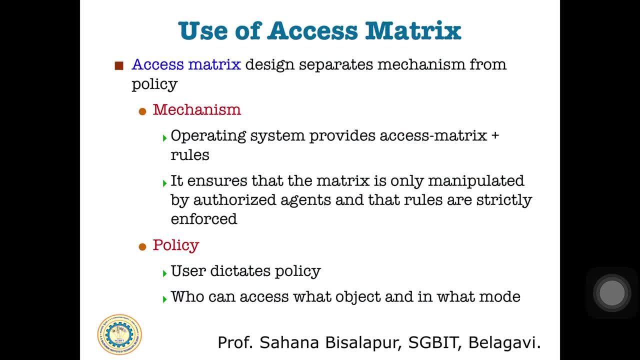 allowed by the access matrix entries. For example, in previous figure we saw where we had for domain D1 and file F1 we had provided the read operation. So it must have only read operation on that file F1, other than that it should not be permitted for other operations. 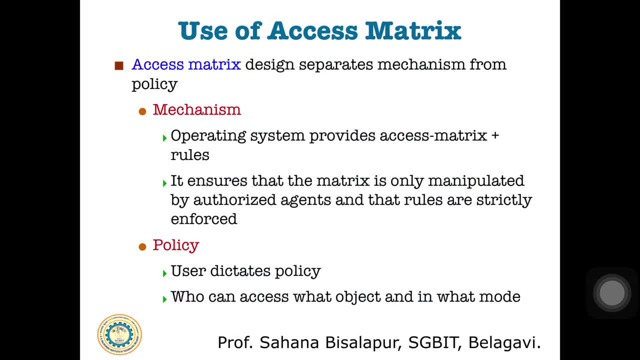 So here We may also, we, we can also implement policy decisions concerned to protection. So the policy decisions involve which rights should be included in the IJth entry. So we are having rows and columns here. So what rights we are going to write here? that completely is decided by using the policy. So 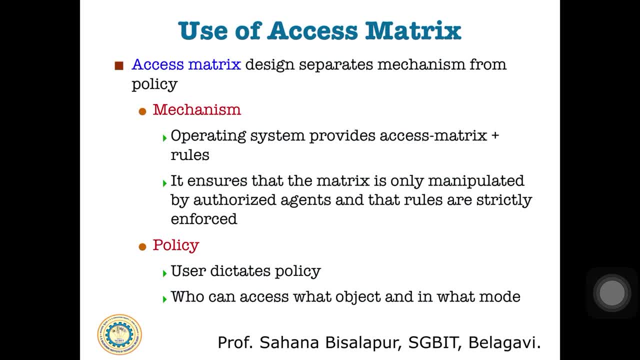 we must also decide the domain in which each process is executing, and here the users are normally deciding the contents of the access matrix entries. So whenever a user creates a new object OJ, the column OJ is added to the access matrix with the appropriate entry made. 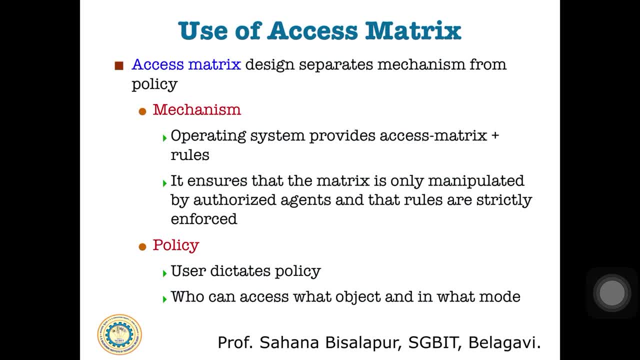 into that particular column. So as the user is the creator, he is going to define the access rights into that particular column. So we can also implement policy decisions concerning that matrix. So the user may decide to enter some rights in some entries in column J and other. 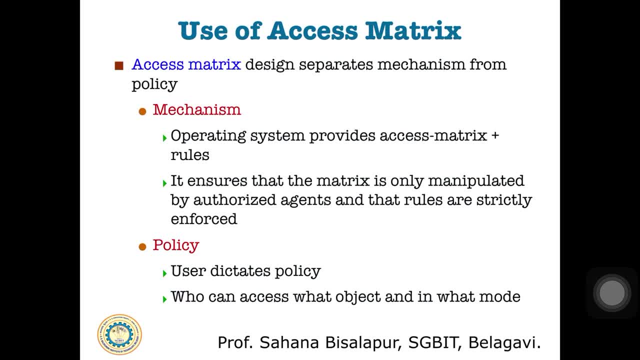 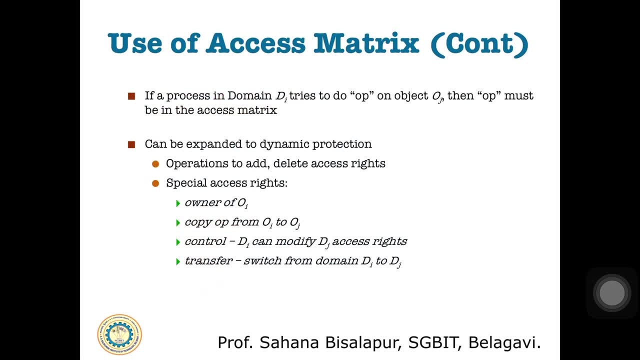 rights in other entries, as it is required. So to continue with access matrix. So here we have to remember that if a process in domain DI tries to do any operation on object OJ, then operation must be in the access matrix. So if a process in domain DI tries to do any operation on object OJ, 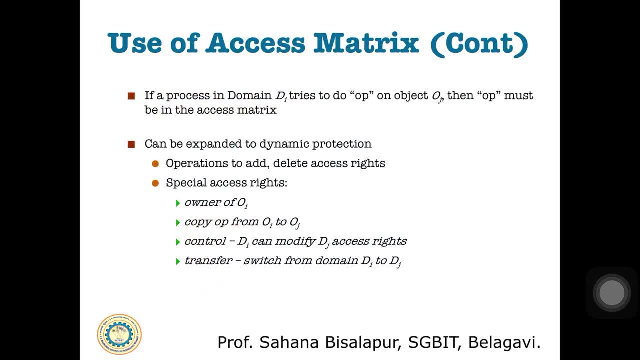 then operation must be defined. If that process in domain DI tries to do any operation on object, so that it tries to do any operation on object OJ, then it has to be property. it ah can be written or used in the type of contentination itself. So if an object, the character you decide, to enter is 0, then you can break it into 2 by test. if you at the and cut, so it will show all certain 7s data. If then you happen to not want to compare, So if the number Dev appetizing, if we go to the, I have to draft and what you need is: the Где you can use the comment, but you should have the moment you are here now in the under row of homework. for that process, though, I should not go through all those C. Поэтому you can simply write the metrics for your file, but you cannot use it. only otherwise you will, unfortunately. 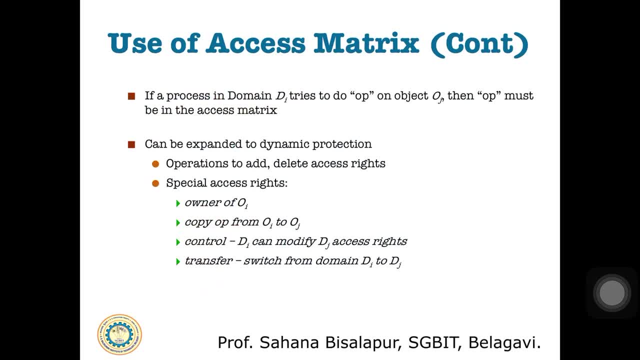 dynamic protection and what all operations we are going to perform. like we can add the access rights, we can delete the access rights and we do also have some special access rights. like we have owner rights, copy rights and control and transfer rights. or we can call: 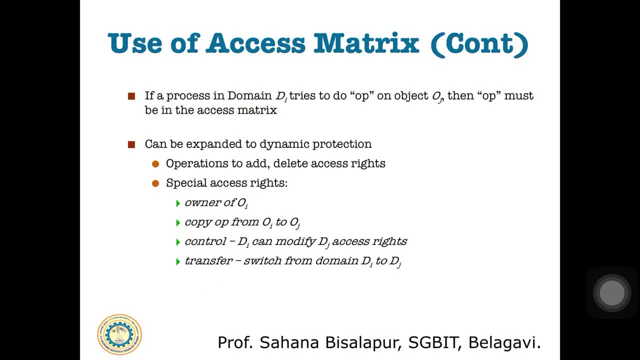 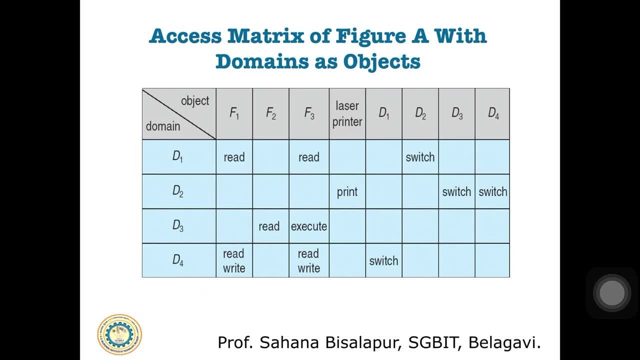 it as switch rights. So we will see these one by one. So first one we will see is with switching. So whenever we switch a process from one domain to another, then we are doing this by performing switch operation on the object. So here the process should be able to switch from one domain to another domain. 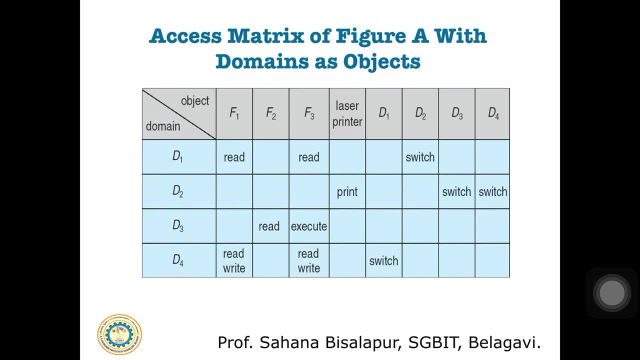 So how the switching can be performed here. So the switching from domain di to domain dj is allowed if, and only if, the access right switch belongs to access ij. Now, as you can see in the figure, it is in the slide- a process executing in domain d2. 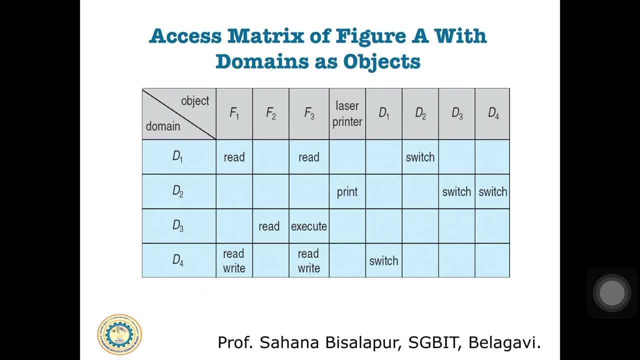 can switch to domain d3 or to domain d4 as we have written in the matrix as switch in that particular entry And a process in domain d4 can switch to d1. Or one in you can say one in one process in domain d1 can switch to d2.. 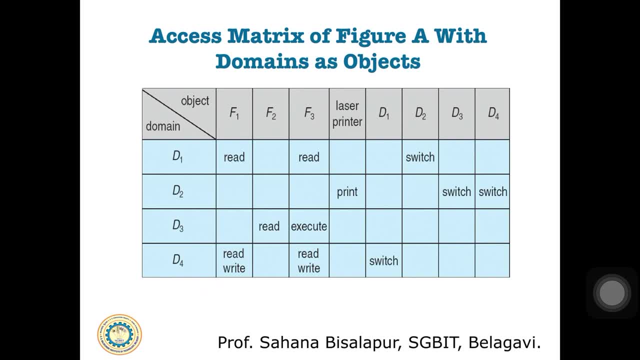 So here you can transfer the processes from one domain to another domain here by allowing the switching operation, or it can be also called as transfer operation, that is, from one domain to another domain, And we can also allow the control change in contents of the access matrix entries, which 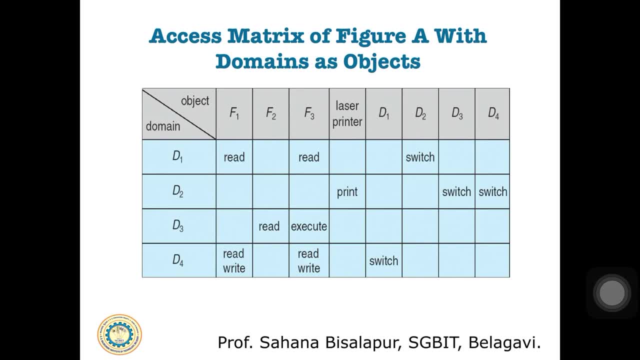 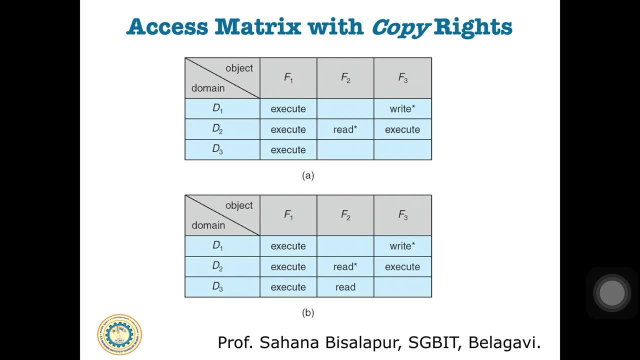 are done by the domain And by using the another three operations, that is, copy, owner and control. So those we are going to see further. So first we will see access matrix with copyrights. So here the ability to copy and access right from one domain, that is, from one row of the. 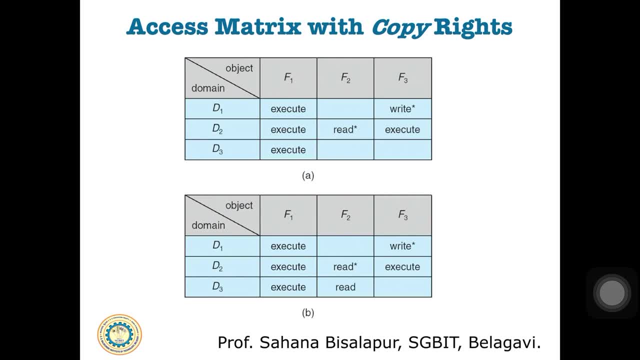 access matrix to the another is denoted by asterisk mark or in the common language we call it as a star mark, Which is appended to the domain. You can see in the slide in figure a and b we are having a star mark with read and write. 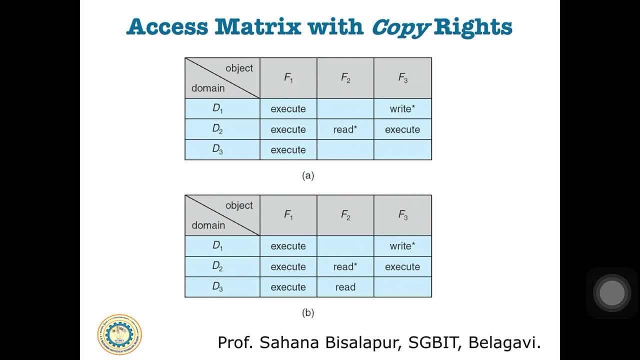 operation in a figure and same with b. So here the ability to copy and access right from one domain to another domain of access matrix which is denoted by an asterisk mark. So here the copyright allows the access right to be copied only within the column for which. 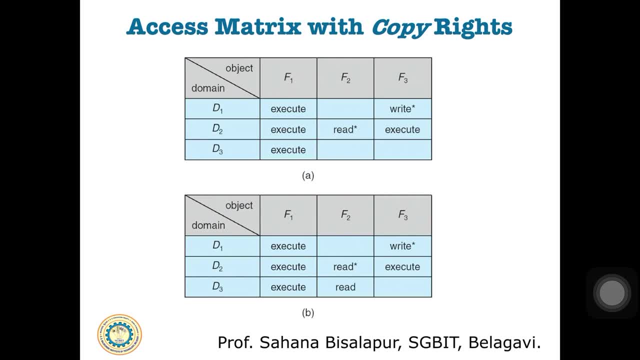 the right is defined. That means you can't just shift it throughout the rows, You can just change it through among the same column here. So you can just consider an example by seeing the figure. So here a process executing in domain d2 can copy the read operation in any entry associated. 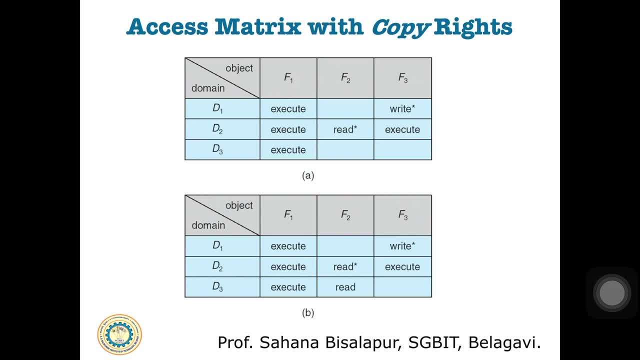 with file f2.. So as you can see in figure a, d2 is performing read operation on f2. And it is marked by star. That means you can perform copy operation of this read operation into any associated column. That means in the same column concerned with only file 2, you can copy it into other domain. 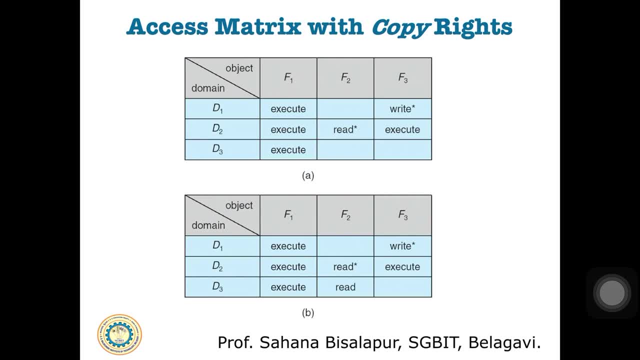 So here. hence it can be modified to the access matrix which is shown in figure b. You can see in figure b The same read operation: it is copied into domain. So that's all, guys. but it is not having a star mark there. that means it cannot be further copied there. so that's it. 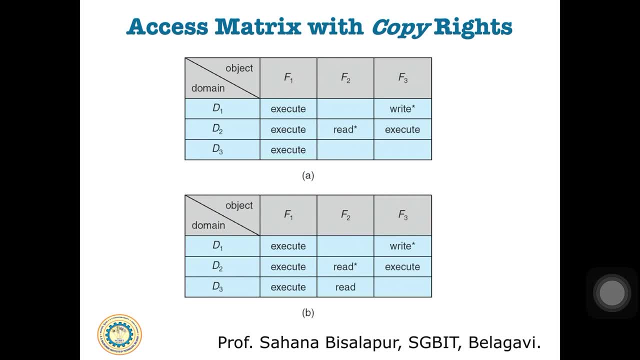 you have just performed one time copy. only domain d2 can perform the copy into the other domain. so this scheme is having two variations here. so one is right- is copied from access ij to access kj. so here you can consider access 2. 2 that means domain 2, file 2, and it is copied into domain. 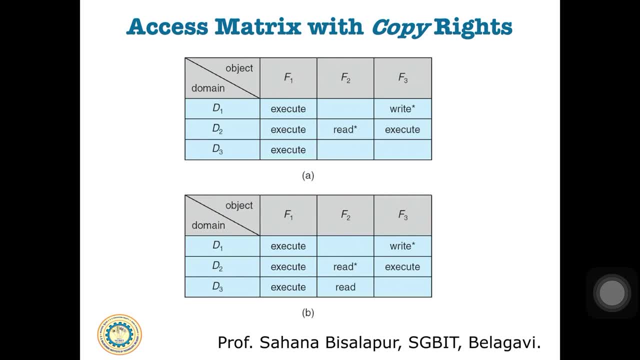 3, 2, that is domain 3, file 2. it is then removed from access ij. so here you are performing the transfer of a right rather than copy. now, for example, if you just copy, move this: read from d2- f2 to d3 f2 completely. 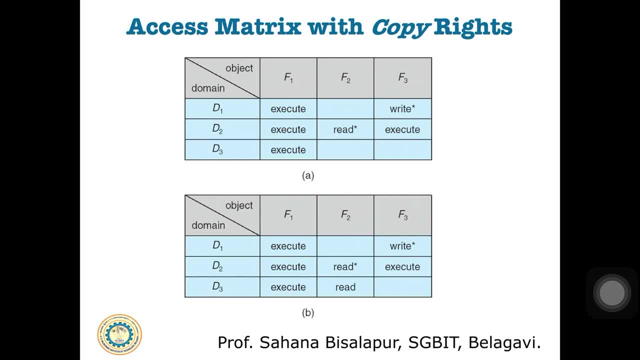 then you are performing transfer operation here, But here what we are doing, we have D2F2 read operation as it is and you are also copying into D3F2, right? So here what we are doing, we are just propagating this copyright, that is, we are just propagating this read operation. 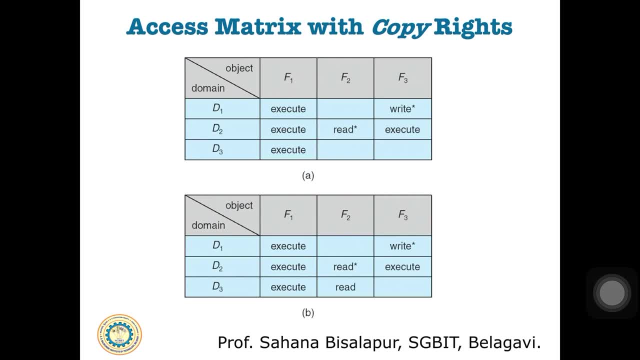 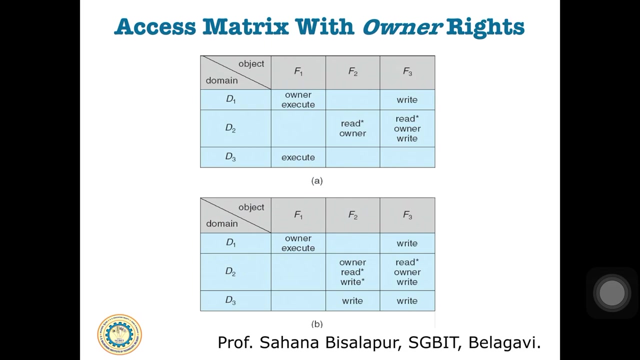 into the other domain. So this operation is called, as here, copying the writes from one domain to another domain. So here we also need some mechanisms to allow some addition of new writes or removal of writes from the rows, So that we are going to see here, So here who can do this. 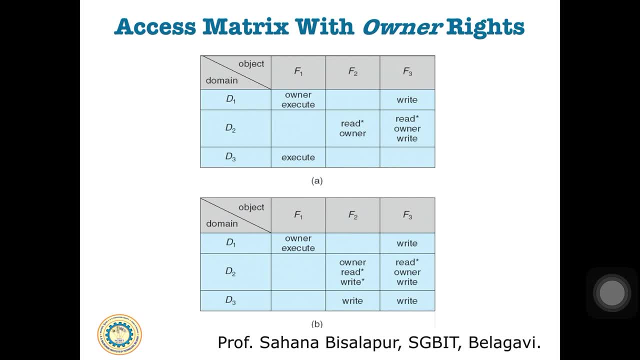 who can add the new access writes and who can remove the writes. here it can be done only by the owner. So that is, we are going to see through this. that is So the owner write controls these operations here. So if the access IJ includes the owner, 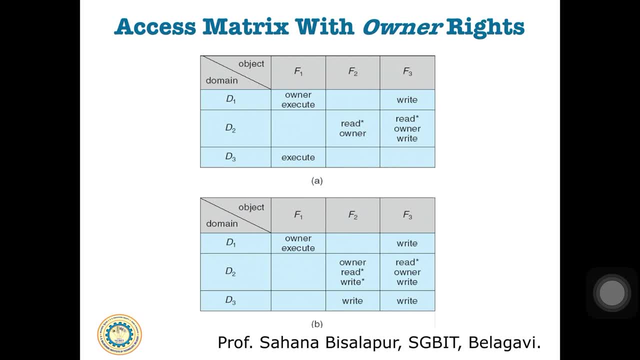 write, then the process executing in domain DI can add and remove any write in any entry in column J. So example we will consider here is: you can see here the figure A. So domain D1 is owner of F1.. You can see we have written the access, write as owner and also execute, right. So here D1 is the. 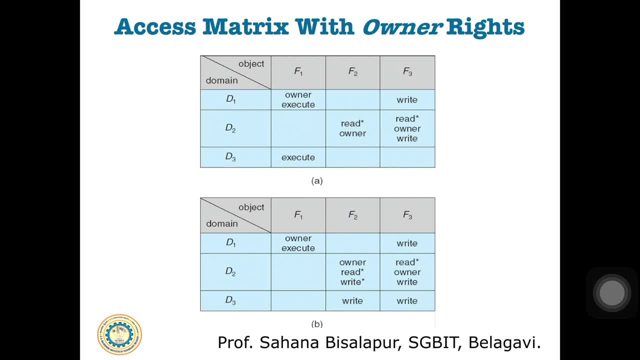 owner of F1, and thus D1 can add and delete any valid write in column F1.. So he can just perform any addition or deletion of writes in this column. that is for particular file F1.. So similarly D2 is the owner of F2 file. So here D1 is the owner of F1. So similarly D2 is the owner of F2 file. 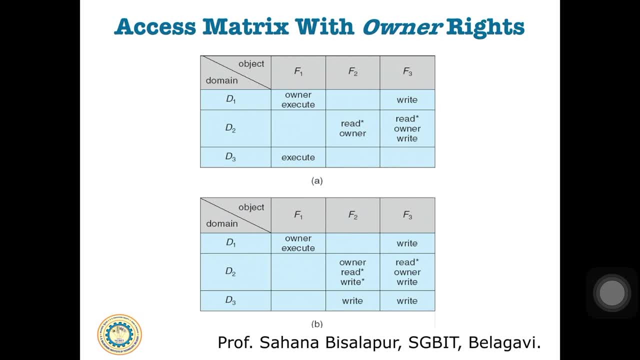 And F3 file and thus can add and remove any valid write within these two columns. So thus the access matrix, which can be modified as shown in figure B- Here you can see the copy and owner writes- allow the process to change the entries in the column. Now here we have changed the 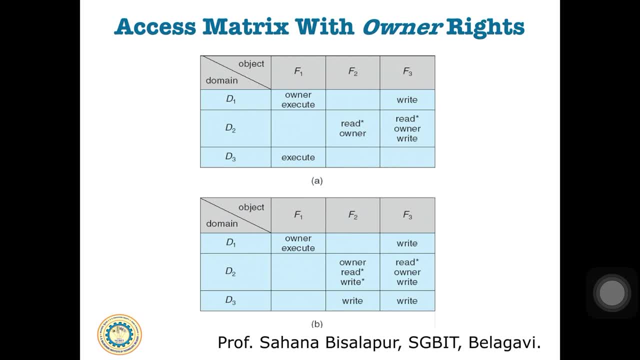 entries in the column. Now, for example, in figure B, D3 has lost the rights of to execute the file F1. So as a owner, D1 has removed that write from D3.. And D2 as a owner for file F2 and. 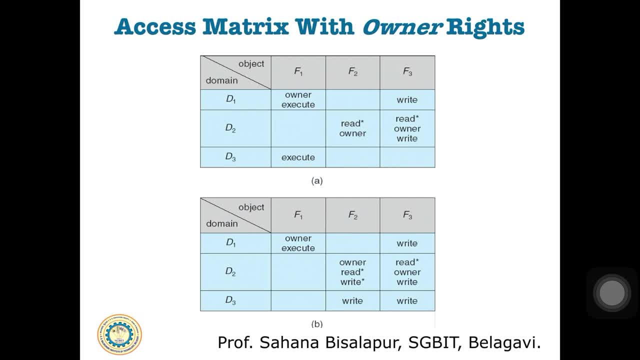 F3, he has added one more operation, that is write operation, which can be copied to other domain. Yes, as it is marked with star. So here D2 can. D2 has added write operation to into file F2, that is for domain D1.. So here D2 has added write operation to into file F2, that is for domain D1. 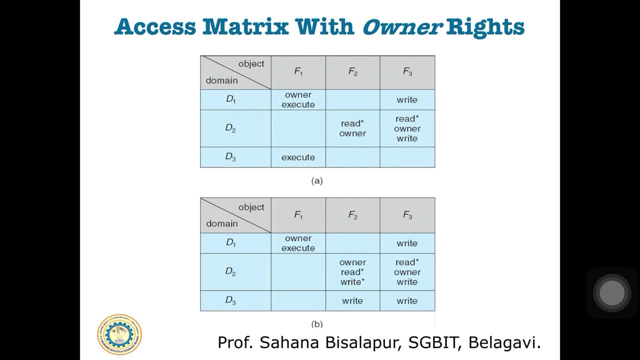 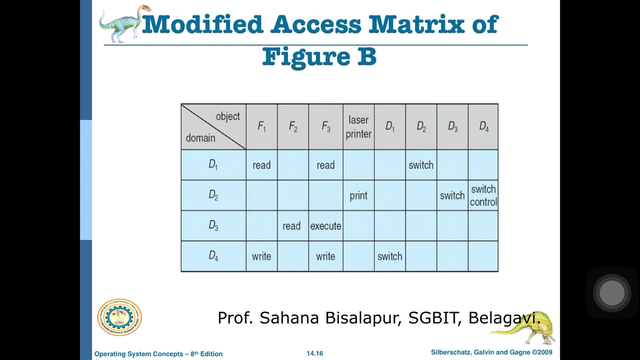 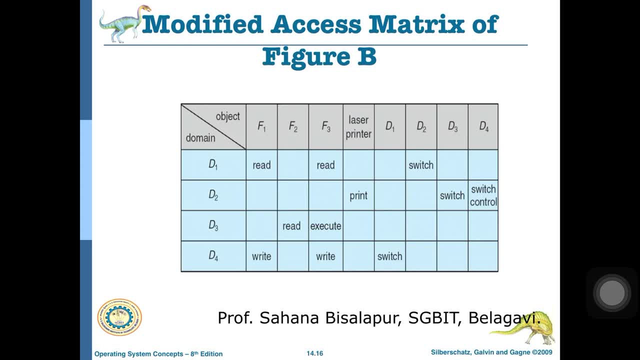 can be done. So now what we saw. We saw how a copy operation can be done. So now what we saw. We saw什 how owner can add or delete the entries in the access matrix And copy operation. and the owner. 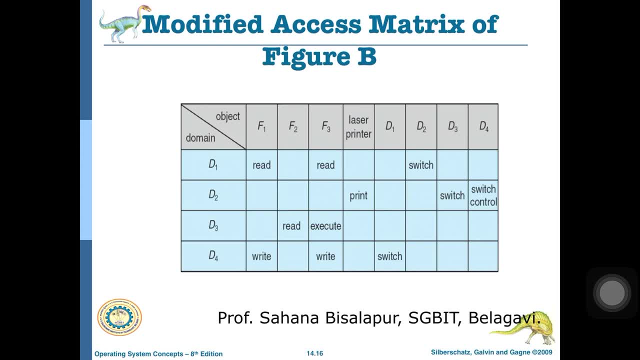 operation, that is, add and delete operation, were done only in the column. We were not supposed to do row wise, Yes. So here we will also see the another mechanism which is also needed to change the entries in a row. So we just now saw the entries which were changed in the column. 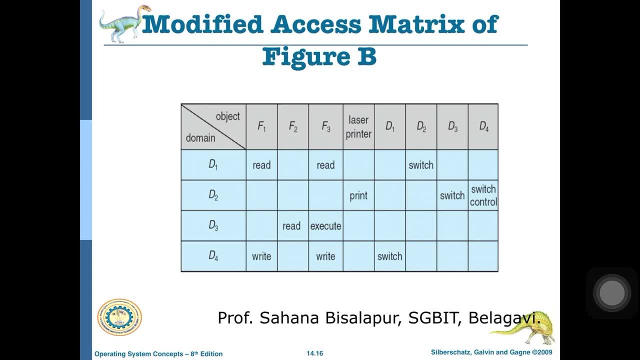 but now we will see the changes that we can make to the entries in a row. So this is done by control right. So here the control right is applicable only to the domain objects. So if access i j includes the control right, then a process executing in domain d i can remove any.